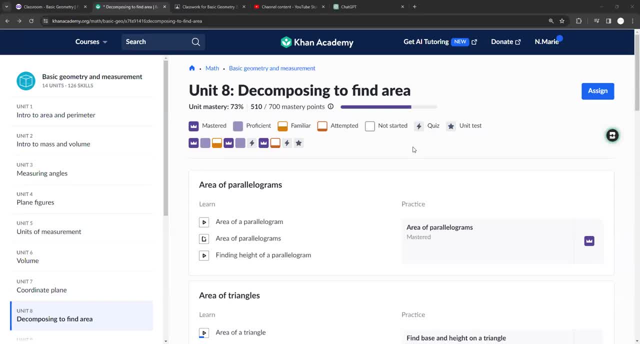 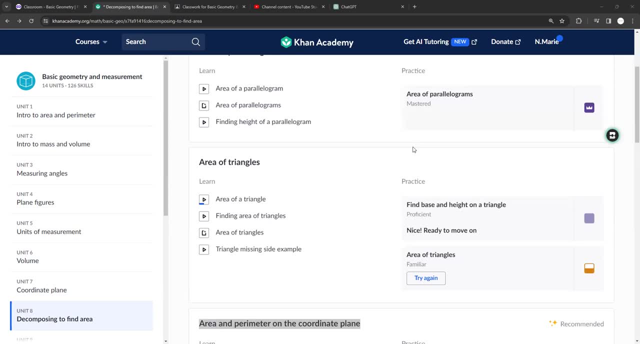 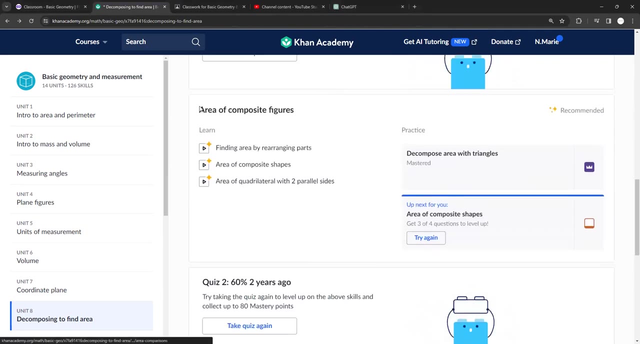 Okay, so in this video we are going to be doing unit eight on Khan Academy, which is decomposing to find area. So we'll be finding area of parallelograms, triangles, and dealing with area and perimeter on the coordinate plane which is up to quiz one, and then area. 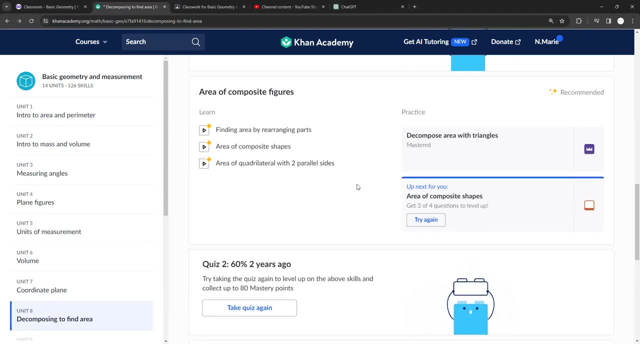 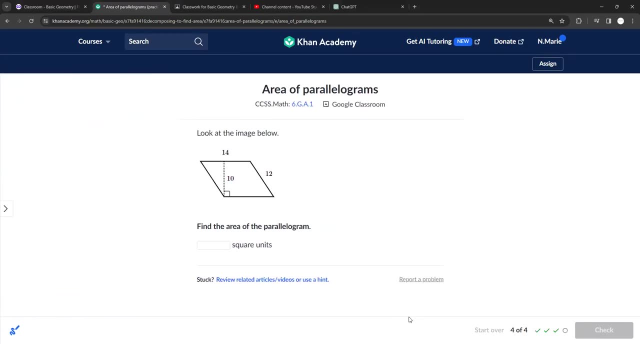 of composite figures up to quiz two. And that's the remainder of this unit. I will be splitting it into two videos. So parallelograms have four sides. So opposite sides for parallelograms are parallel And since it's a quadrilateral it has four sides and it equals the internal sum of 360. 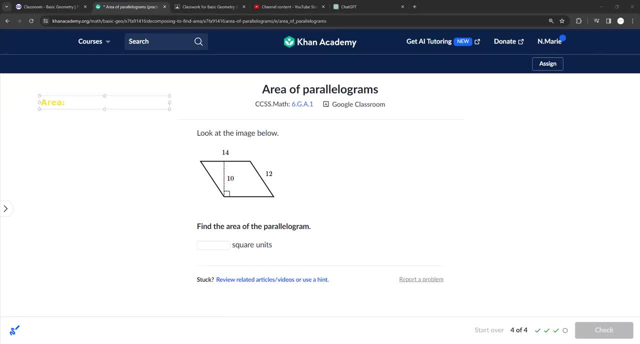 For parallelograms the area formula is base times height. Base and height will always be perpendicular to each other. with shapes This is the same for triangles when we do them next. So you can see here: height is how tall a figure is and then base is the bottom. you can see that. 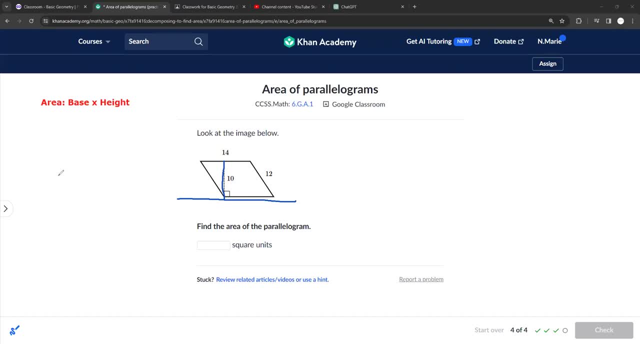 90 degree angle. there They are always perpendicular base and height. So make sure you're careful with these. A lot of times students mess up. they don't know which is the base and which is the height For parallelograms. opposite sides are equal, So if that's 14, that's 14.. If that's. 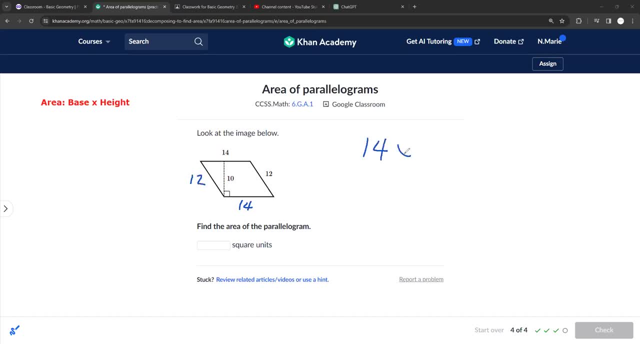 12,, that's 12.. So the base would be 14,, the height is 10.. And then we would multiply that and divide by two. 14 times 10 is 140.. Divide that by two And you would get 70. So the area which is the inside of the shape. Wait, hold on. I think I. 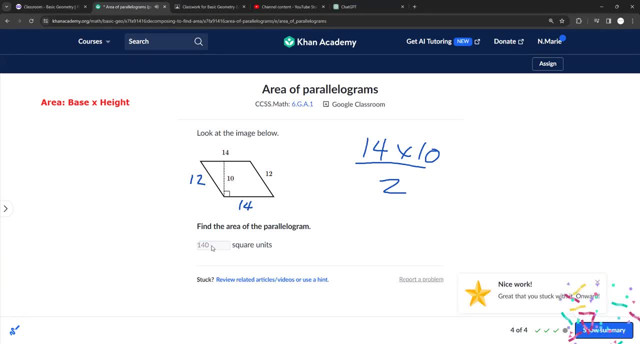 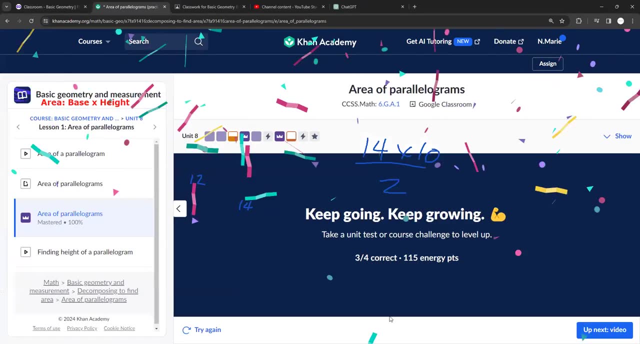 oh sorry, Why did I divide by two? Ignore that, Just base times height. Sorry, I'm thinking of triangles. For triangles it's base times height divided by two, So you would get 40, for this one 140.. So the parallelograms are pretty easy. You just do base times height, So careful. 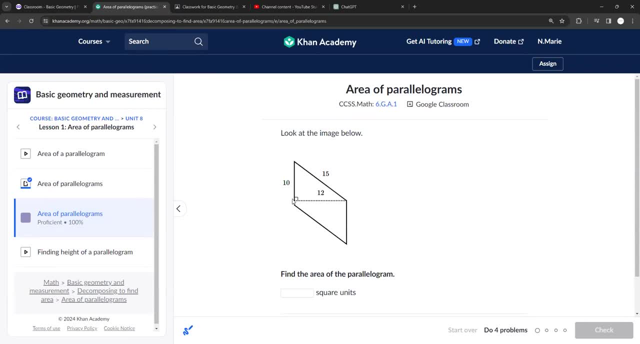 which is the base and which is the height For this one. if this is the height, which is 12,, the base is 10.. So it'd be 120.. For this one, the height would be 14.. The base is six, So 14 times six would get you the. 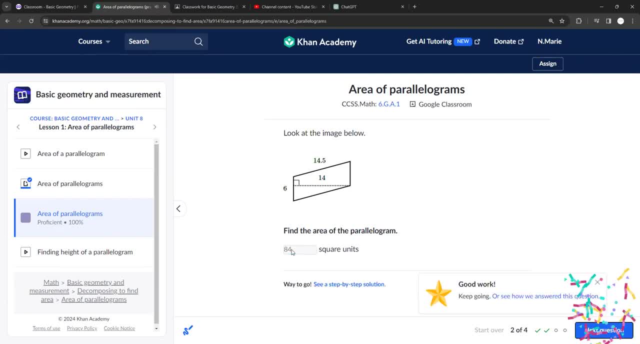 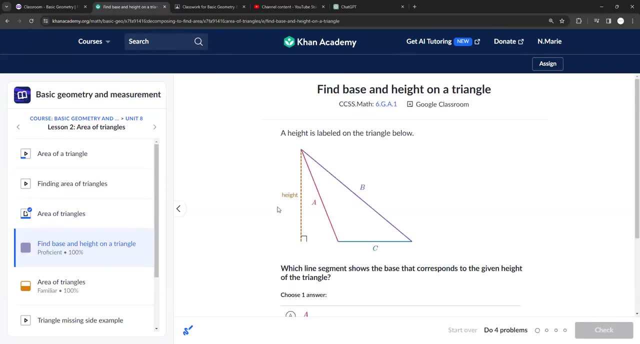 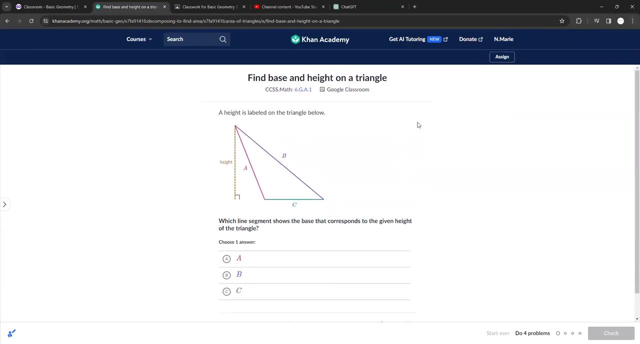 area, which is the inside space of the shape, And so on. These are pretty simple to do. Triangles are a little difficult sometimes for students only because they have trouble correctly identifying what's the base and what's the height. Okay, so if this is the height, the base has to be. 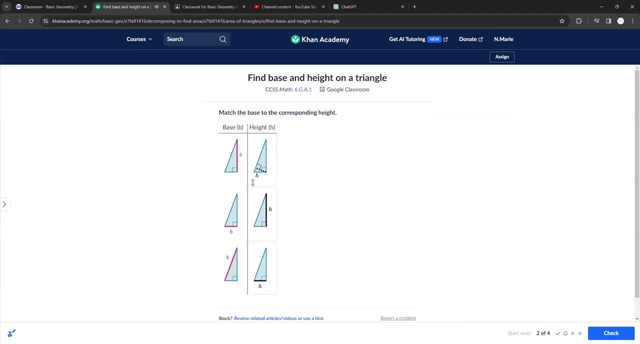 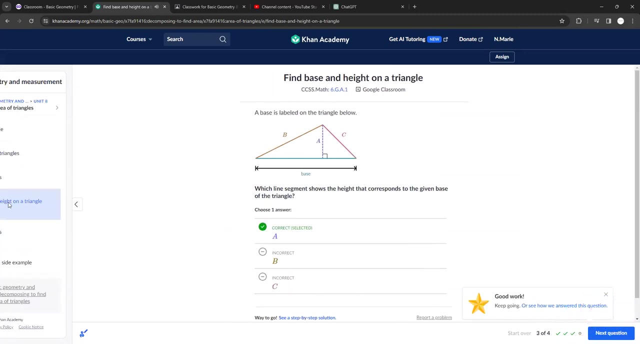 perpendicular, So it would be C. So these you can see, they're having you match up the height with the base. So remember, find the one that's perpendicular And then we'd match them up. If this is the base, A is the height. So they want you to go spend time practicing. 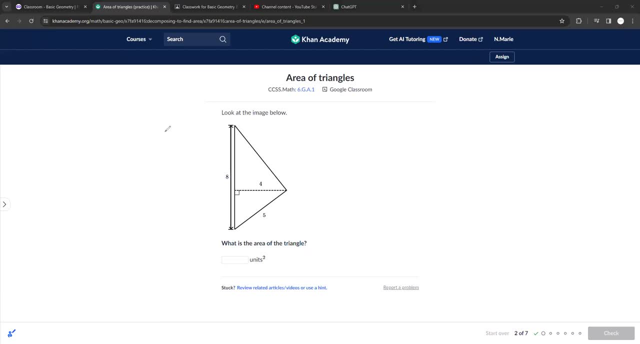 doing base, finding the base and the height, because you want to be able to do that correctly when you find the area of a triangle which is base times height divided by two. So, and the reason is because you know this is not a full shape, right? If I were to make this a? 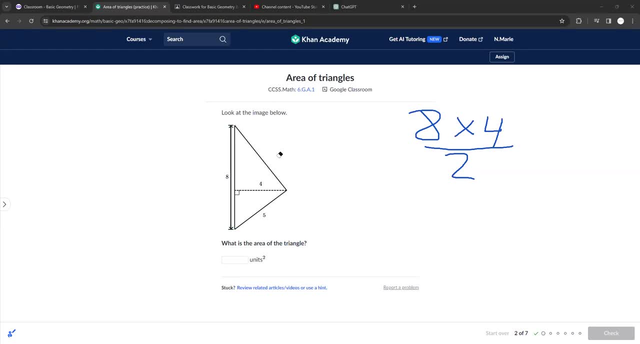 full shape. that would just be length times width, base times height. But since triangles are like half of rectangles, you split it in half. Okay, so that would get us 32 times 32, divided by two, which is 16.. So here we would do 21 times six, which is 126.. We would divide that by two and we 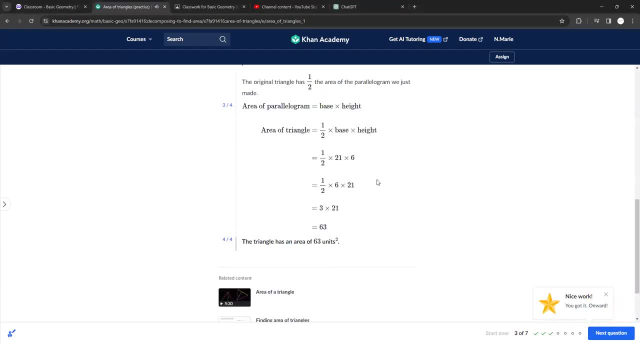 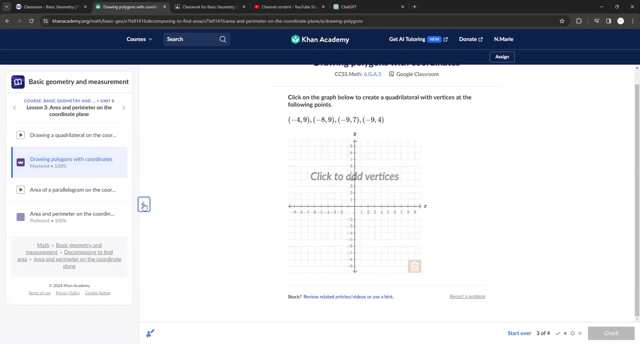 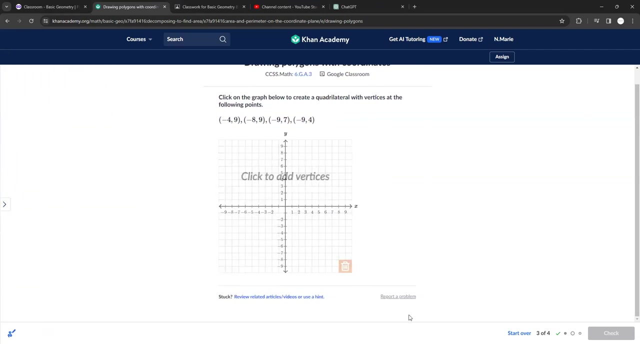 would get 63. So make sure you practice Doing area for triangles. You can also do one half times base times, height, same thing, get to the same answer. Okay, so doing these on the coordinate plane. So let's plot the points. This is at negative four nine. So remember the coordinates are. 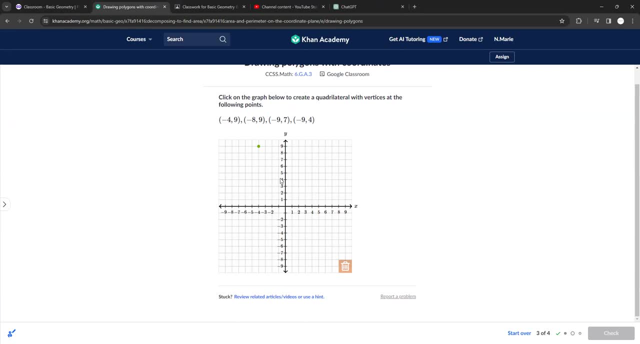 plotted X before X, So let's plot the points. This is at negative four nine. So remember the coordinates are plotted X before X, So let's plot the points. This is at negative four Y. We've done the coordinate plane in previous units, so we should already know how it works. 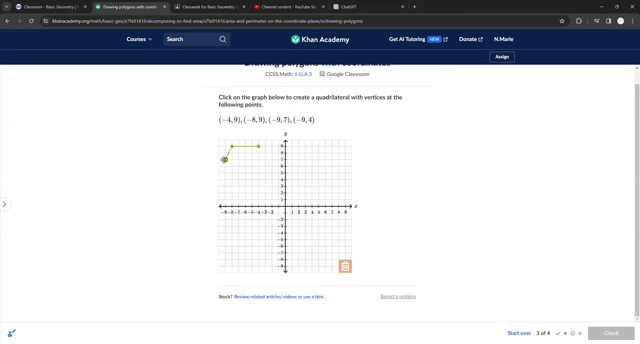 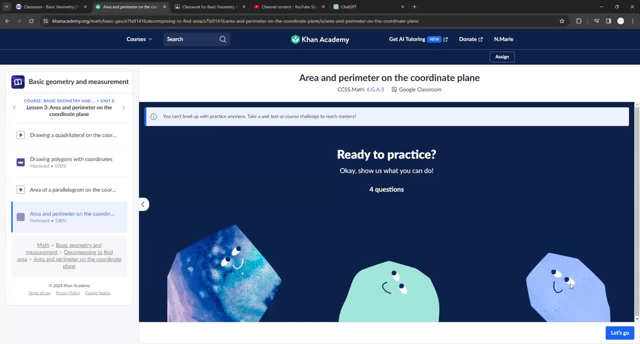 yeah, Definitely. it's in my mens cancel form. So what you want to do is just place it and you contract the first one, You fabulous. And so it creates like a little hierarchy첀. What about having a pointer simply disadvantages? 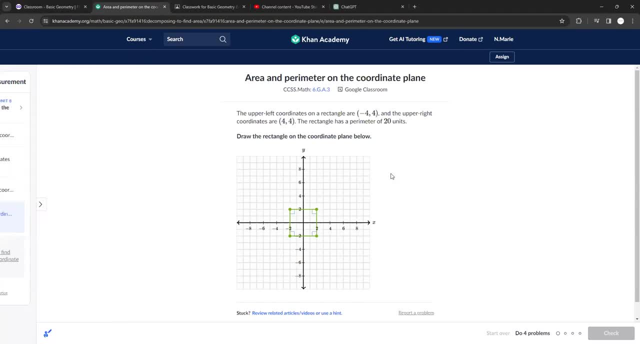 So what you want to do, It's just kind of like having one but it's a little add two. There's now something to perfect it, but that would be really good to do if you want to be sophisticated with it, to make it something that is important. 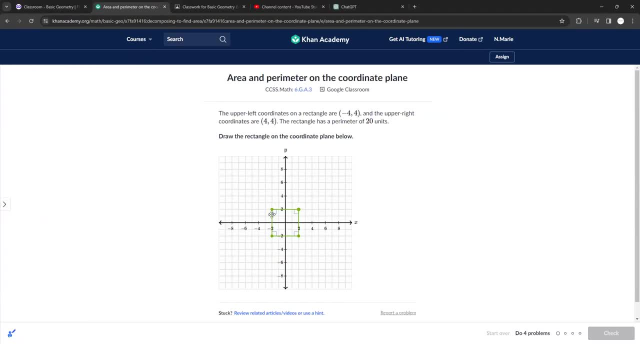 Last but not least, just actually finish this: Theseeu过 or at. so the upper left coordinates is at negative four, four. The upper right is at four, four, And it says that the perimeter is 20 units. Okay, So right now, this is one, two, three, four. 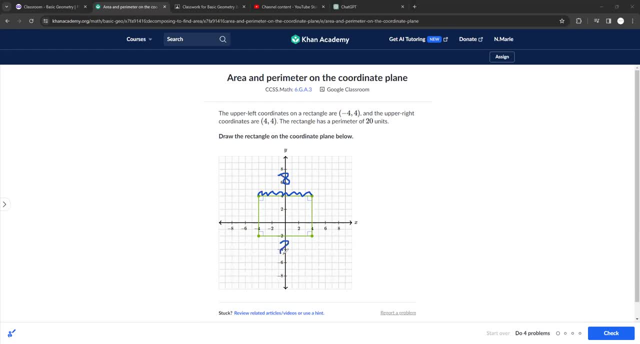 five, six, seven, eight units, And so that means the other side has to be eight. So that already gives us 16.. So remember, perimeter is when you add all the sides. So 16 plus what gets you 20, and that would be 16 plus four. So that means this side has to be two and the other side to be 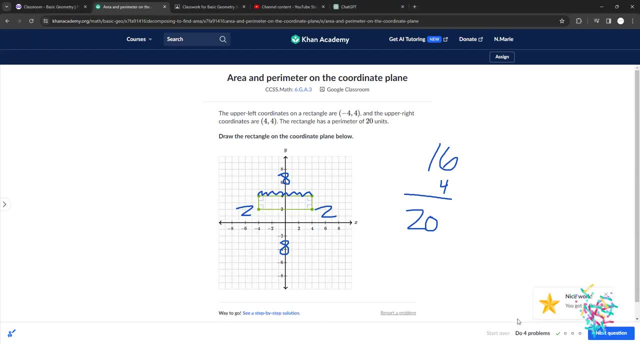 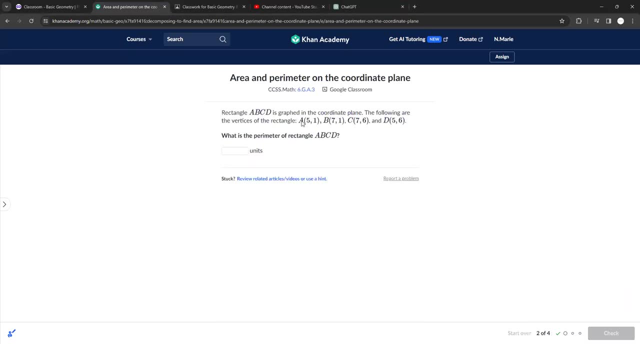 two as well. And so there we would do a rectangle and the perimeter of 20 units. So here you can graph this graphing paper and then you can find perimeter. But you can see. so if we did like, if we were to graph this coordinate plane, 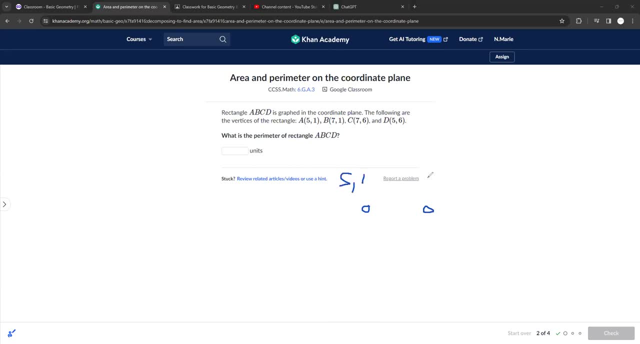 you know it'd be AB, So this would be five one, seven one. So you can see. the distance from this is only two, right? How do I get from five to seven Two? Is it a rectangle? Yes, Okay. 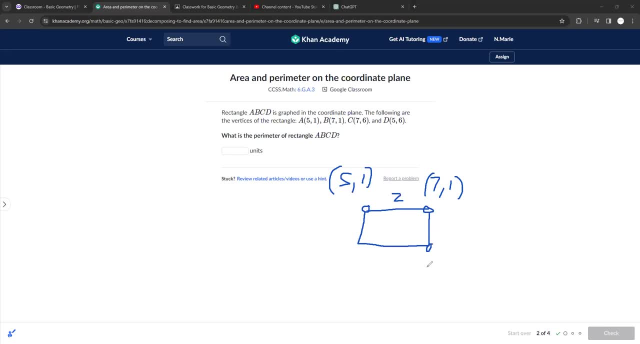 And so this one's at. it should be up actually, but it's okay Actually. yeah, let's draw it the correct way. if we were to put this on the graph, So this would be at seven six and this would be. 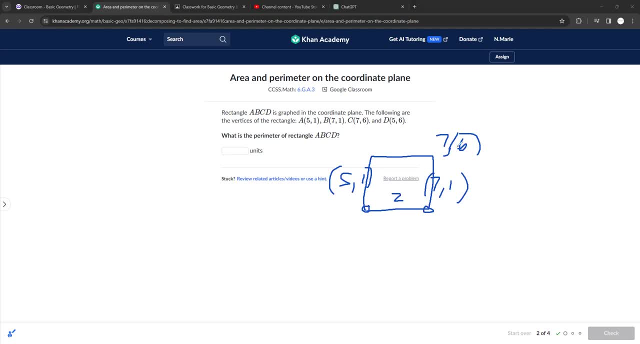 oops, this would be at seven, six, And this would be at five, six, And so, once again, that's two away. And what's the distance from up? So let's just draw it here: This is two, this is two. How do I get from one to six for the? 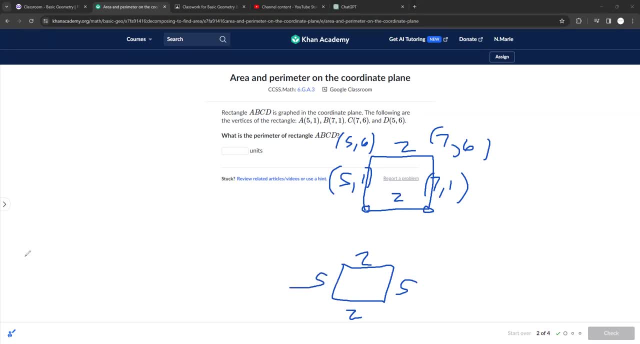 Y values. That goes up five. that goes up five. So there, total of 14 units when you add all the sides. And so for area, you would do the same, You would see. you know what's the distance. 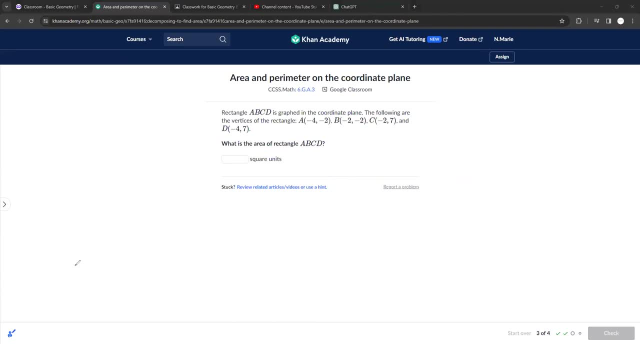 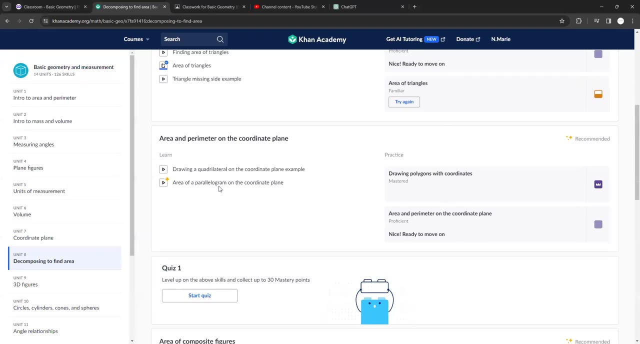 Feel free to graph on graphing paper if you need to, And then for area you do: length times width. So that's pretty much the beginning of this unit. It's very simple. If you have any questions or need additional videos on anything, let me know. Good luck.